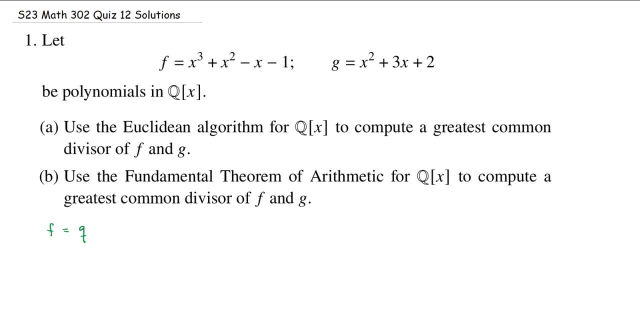 polynomial and I should be able to write F as Q times G plus some R, where the degree of R is less than the degree of G, which in this case is equal to 2. okay, so I'm just gonna copy my F: x cubed plus x squared: minus x minus 1 equals okay, well, 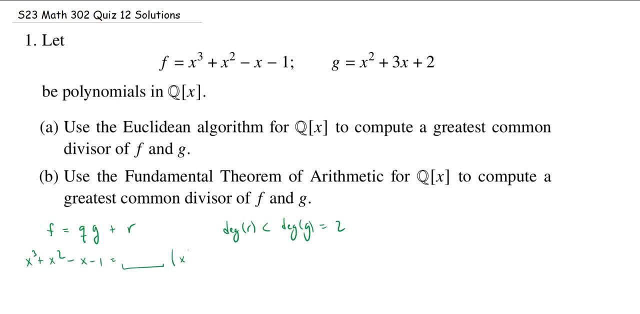 I'm gonna have my Q, and then I have my G, which is x squared plus 3x plus 2, and then there would be some remainder. all right, well, what I do in the first bit is I'm going to basically see what. what can I multiply my G by to get as close to F? 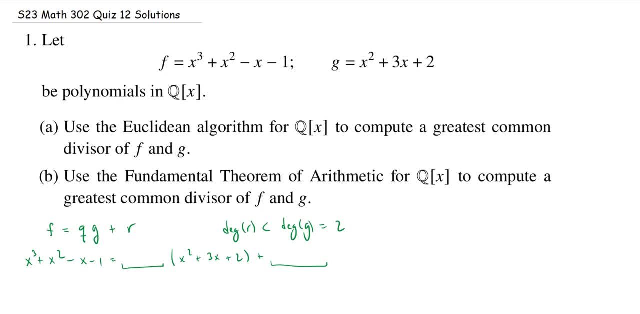 as possible. so, for example, I know I need to get x cubed, but I have x squared. so what if I multiplied by x? so x times x squared will give me the x cubed. so this is taken care of, okay, but putting the X here, it's also going to multiply by 3x, which will give me 3x. 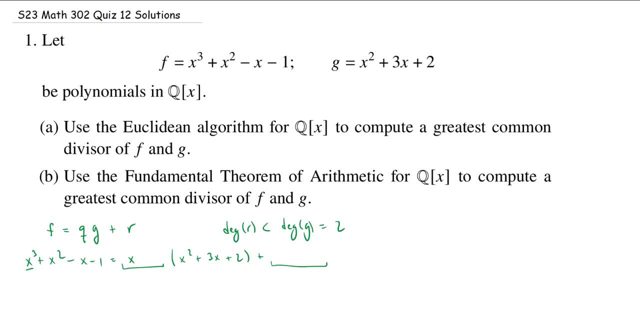 squared, and I don't want 3x squared, I want just 1x squared, so I could get rid of 2 here and now I would have minus 2x squared plus the 3x squared. oh, 3x squared minus 2x squared is 1x squared. okay, that's exactly what I. 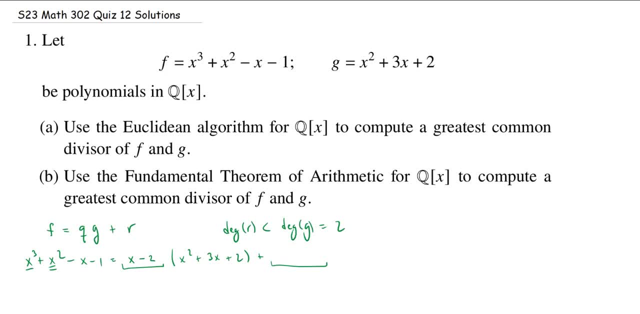 needed, but I now also have x times 2 as well as minus 2 times 3x. ah, so x times 2 is 2x. minus 2 times 3x is minus 6x. that gives me, let's see, minus 6 plus 2 is. 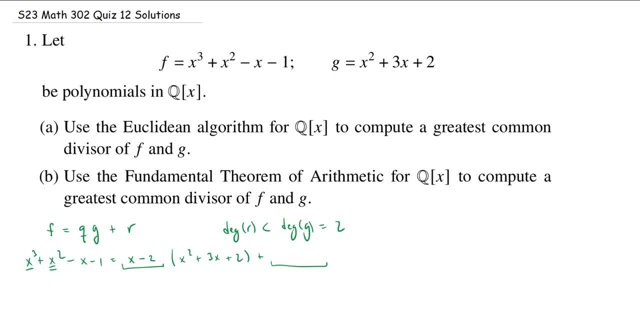 minus 4. so I have minus 4x, but I want minus 1x and you'll notice, here there's there's really nothing left for me to add to do that to this factor, so I'm gonna have to actually include that in the remainder. 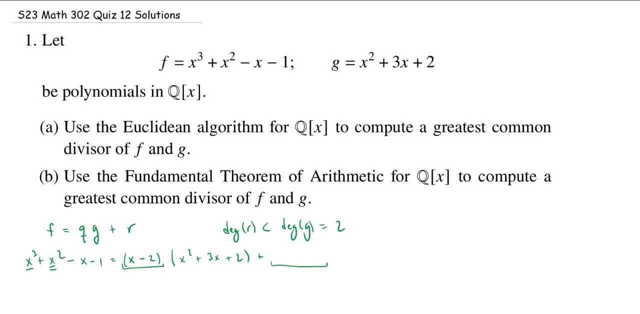 so I have negative 4x. I want negative 1x, so I'm going to add 3x to compensate. all right, I also have minus 2 times positive 2, that's minus 4, and I only want minus 1, so I'm gonna have to add another 3 again to compensate. 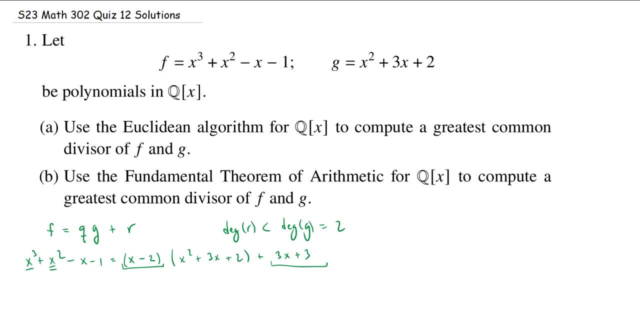 all right. so this is sort of the, the one-line version of essentially doing polynomial division. if, if this is too fast, right, we, you really could, you really could come over here and say, okay, let me do x cubed plus x squared minus x minus 1, and I'll divide by x squared plus 3x plus 2, and we would go through. 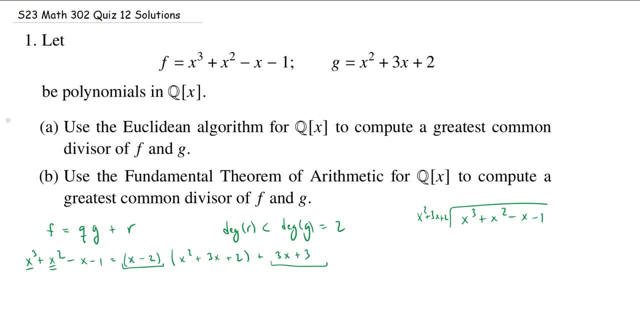 all the usual machinations, right. I multiply x by x squared to get x cubed. and then x by 3x gives me 3x squared. x by 2 gives me 2x. then I subtract and I get x squared minus 3x is negative. 2x squared negative. x minus 2x is minus 3x. 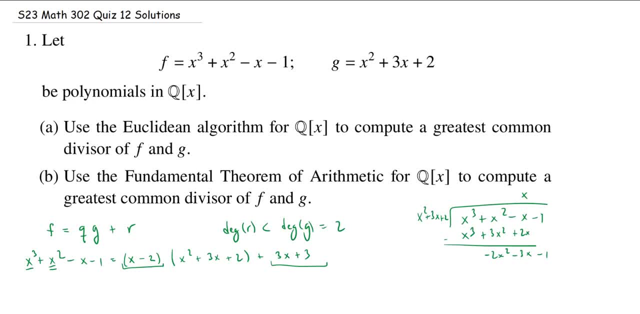 then we bring down a minus 1. hey, I multiply x squared by minus 2 to get negative. 2x squared minus 2 gives me: okay, there's my negative. 2x squared minus 2 by 3x is minus 6x, by minus by plus 2 is minus 4. and then we subtract. and when you subtract, okay, I. 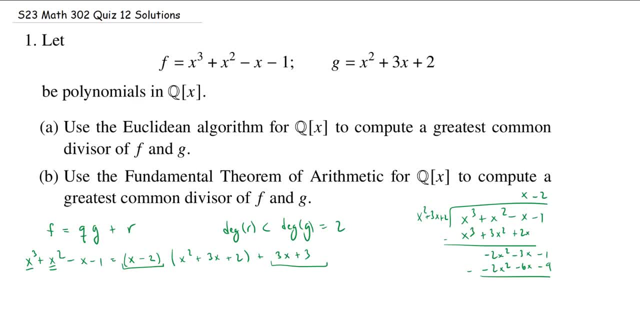 get 0 negative. 3x minus minus is plus 6x, which is 3x negative. 1 minus minus 4 is plus 3. okay, and so we see, we get x minus 2 as our quotient and 3x plus 3 as. 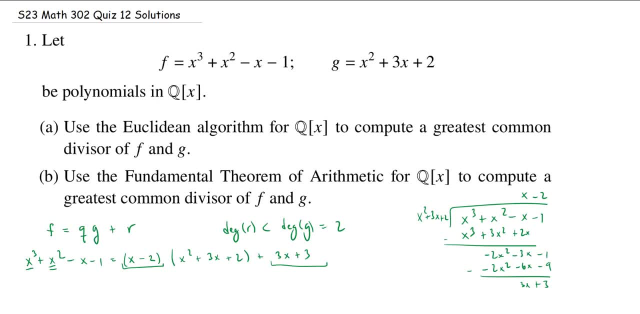 our remainder. okay, so same thing. it's also kind of nice to note that 3 times x plus 3 is the same as 3 times the quantity x plus 1. we'll see in a second why that's going to be a little bit useful now if we want to continue on. 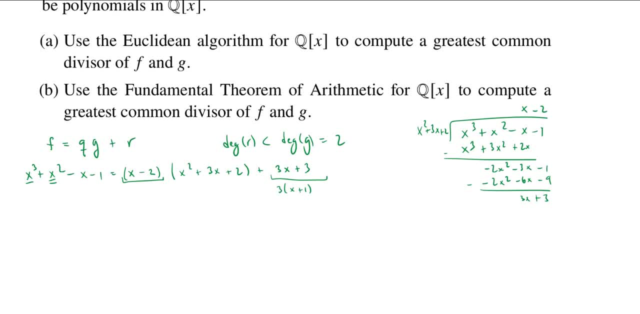 in the Euclidean algorithm, we have to shift the original divisor to become the dividend. the remainder would become the new divisor, and then we get this setup. okay, now I did this little factorizing right: 3 times x plus 1. so instead of dividing 3x plus 3, which is going to give us a bunch of 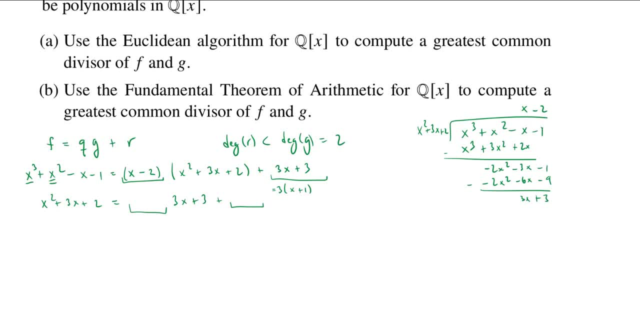 denominators. right, we're going to get a bunch of fractions. I'm just going to divide by x plus 1, and then we can, at the end right, compensate for this, this 3, And this is where it's good to just stop and think for a little second. 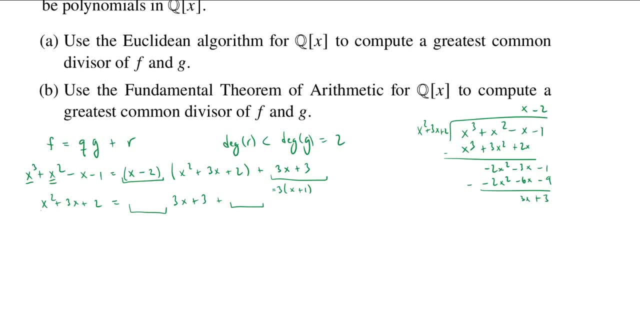 x squared plus 3x plus 2.. I actually can factor that right Like: this becomes x plus 1 times x plus 2.. Or let me write it the other way: x plus 2 times x plus 1.. And then you might say: well geez, I have here 3 times x plus 1.. 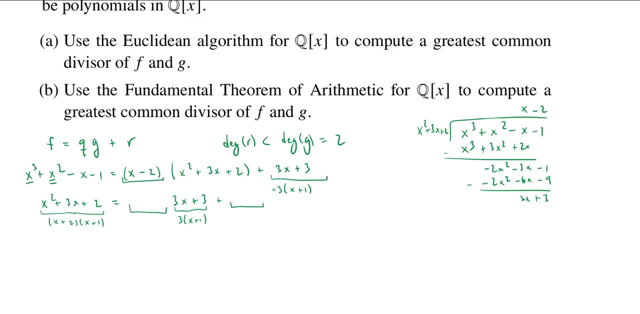 I just need to divide this polynomial by x plus 1.. And I know that's just going to cancel this x plus 1.. And so I would get x plus 2, except, well, I've got to compensate for this 3.. 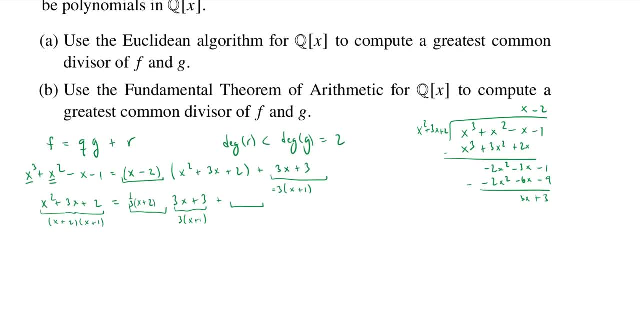 So I could just put a 1 third in the front. Now, of course, you could go and do this without knowing this factorization. You could do long division again. You say: OK, I'm going to take x squared plus 3x plus 2, divide it by well. 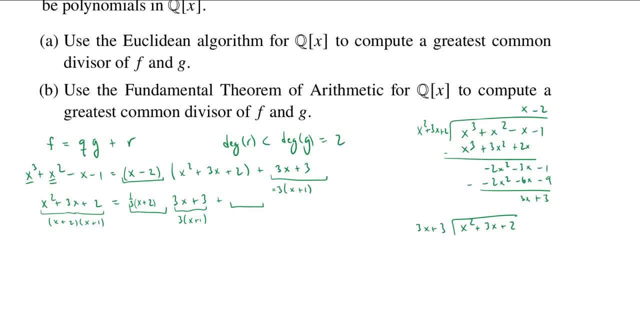 you could even 3x plus 3 and feel really bad about life and say, OK, this is going to be 1 third x. 1 third x by 3x is going to give me x. squared, 1 third x by 3 is going to give me x. 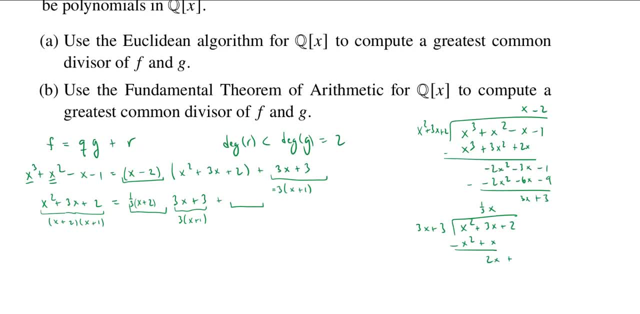 I can subtract and I get 2x. Drop down the 2.. Oh, what do I multiply? Oh my goodness. Well, let's see, If I multiply by 1, third, and then by 2, I'll get 2.. 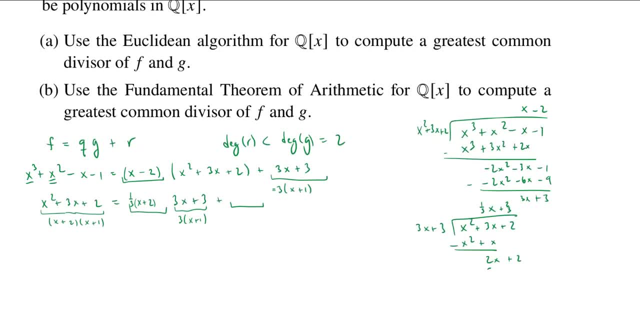 So 2 thirds, All right, so that gives me 2x. And then, hey, 3 times 2 thirds is also 2. And I get no remainder. All right, and so I could factor out 1 third from this. 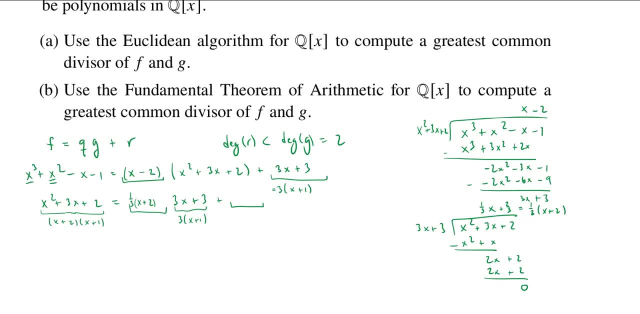 and think of this as 1 third times x plus 2, which you see, is what we get on the left. Also, notice, because it divided evenly, we get no remainder, which means we actually don't need this step right, This is the superfluous division like a divide step. 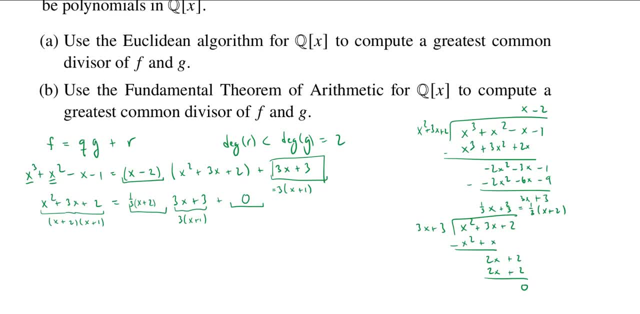 And so the Euclidean algorithm tells us we can use the last non-zero remainder, which we can either take here as 3 times x plus 3, or we could even ignore the 3 and just write x plus 1.. Totally up to us. 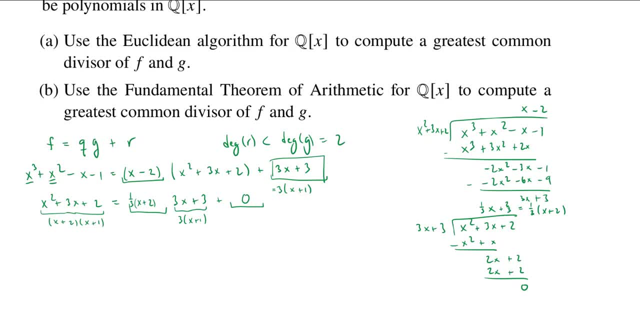 Greatest common divisors are only defined up to multiplication by a unit. So in any case we get that the AGCD of f and g is equal to 3x plus 3, or, if we like, x plus 1,. that's fine too. 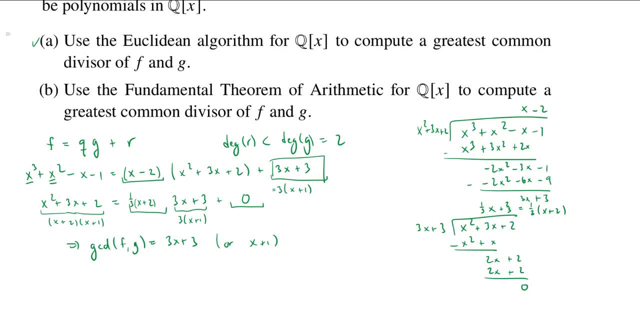 All right, so that's how we handle finding the GCD using the Euclidean algorithm. All right, now what about the fundamental theorem? What about the fundamental theorem of arithmetic? So for the fundamental theorem of arithmetic, we rely on knowing we can take every polynomial over qx. 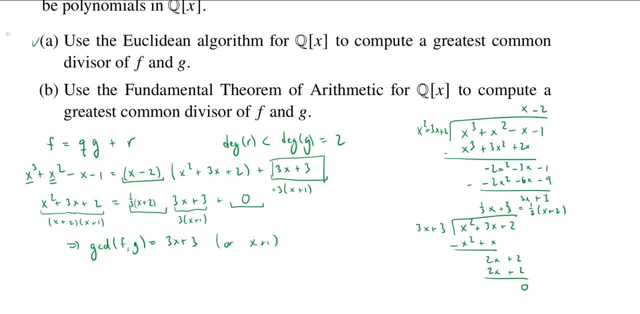 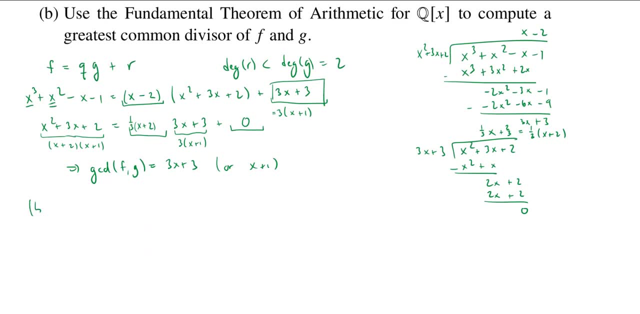 and write it as a product of indecomposable or, if you like, irreducible, polynomials. So we've already actually factored x squared plus 3x plus 2.. So we know that factorization. What about the f? So this was x cubed plus x. 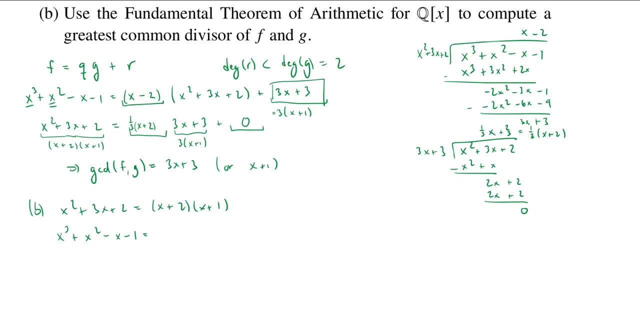 x squared minus x minus 1.. All right, so we could use the rational root theorem here in order to try to find a linear factor. And so we notice the coefficients are 1 and negative 1, so we should really just try the roots 1 and negative 1.. 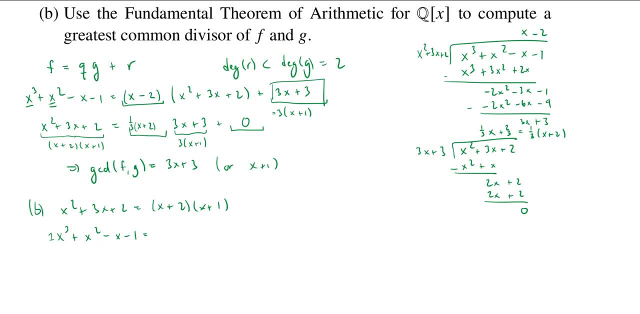 And, sure enough, when I evaluate at 1, I get, let's see, 1 plus 1 minus 1 minus 1 is 0. So actually I will get a factor of x minus 1.. Okay, Let me try negative 1.. 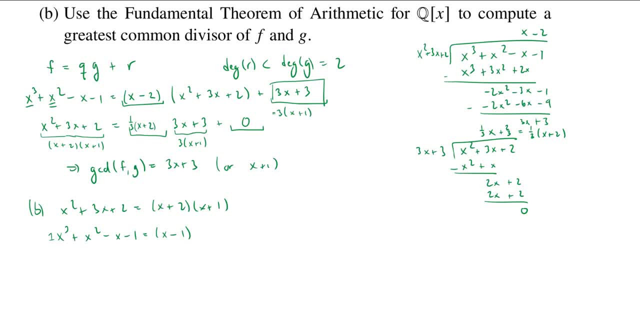 I get negative 1 cubed, which is negative 1, negative 1 squared, which is positive 1.. Okay, so so far I have negative 1 and positive 1.. That's 0.. How about here? Negative, negative 1 is positive 1.. 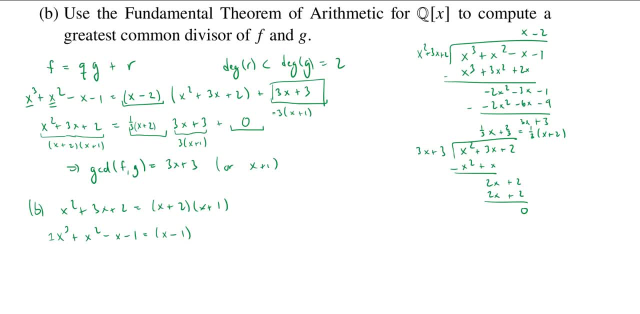 Minus 1 is 0.. Oh, so negative 1 is also a root, And so I know that I have another factor. All right, well, what's left over? Well, we could Try guessing at it. or we could say: well, okay. 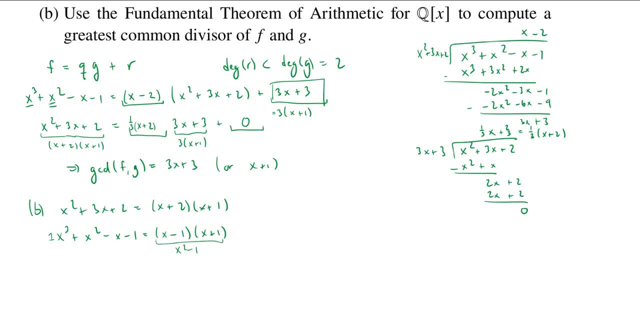 I know this is already x squared minus 1, so let me just divide And I'll say: all right, what do I multiply x squared minus 1 by to get x cubed plus x squared minus x minus 1?? Now I know I would have to multiply the x squared by an x to get x cubed. 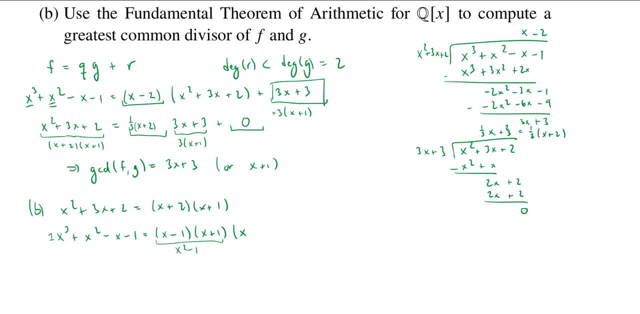 Okay, but then I'm going to get also a minus 1 by x. That's negative x, Negative x. And well, that's actually okay, right, Like I'm supposed to have a negative x, But I'm also supposed to have an x squared. 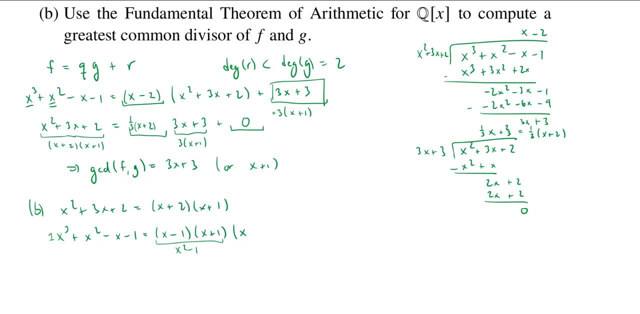 Ah yeah, And here I don't have an x squared, So to get an x squared I could put a plus 1.. Okay, so let's see, Does that mess anything up? I already have my x cubed. Now I have x squared by 1 is x squared? 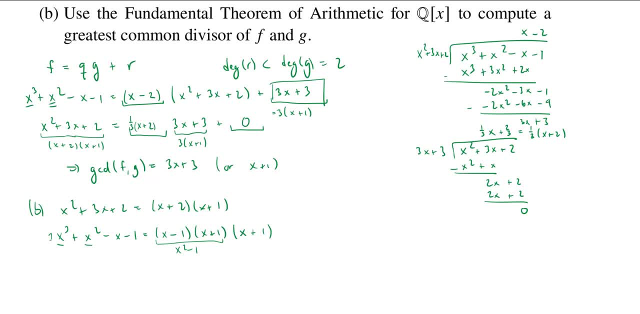 I also have minus x, Because minus 1 by x- Hey, I wanted that- And I have- minus 1 by 1- is minus 1.. Oh, my goodness, I got everything. So in fact, ah, there's just two copies of x plus 1 squared. 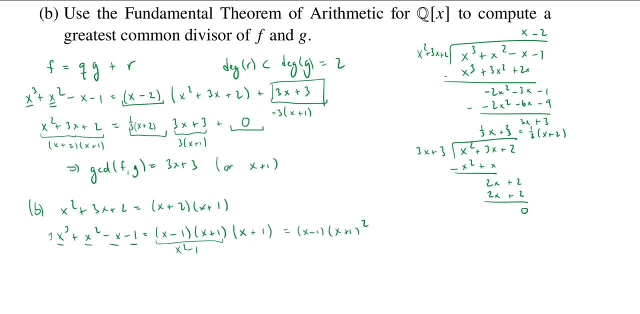 So if I wanted to write it in that more condensed form, I could do so. Okay, so we have factorizations into indecomposable polynomials. Now, the greatest common divisor we can find by choosing each of these irreducible polynomials- or indecomposable, whichever you like- and taking the minimum exponent that occurs. 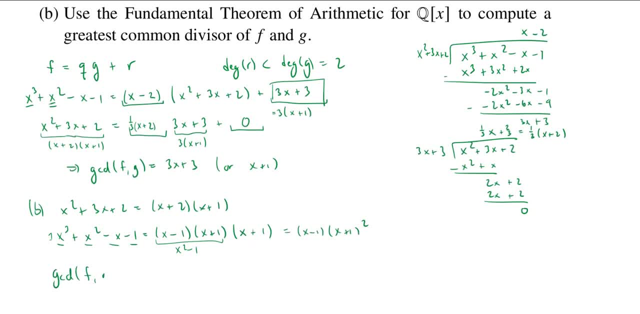 So, for example- all right, we'll set this up- gc, d of f and g I'm going to take. well, let's see, We have 1, the x minus 1, 2, the x plus 1, 3, the x plus 2.. 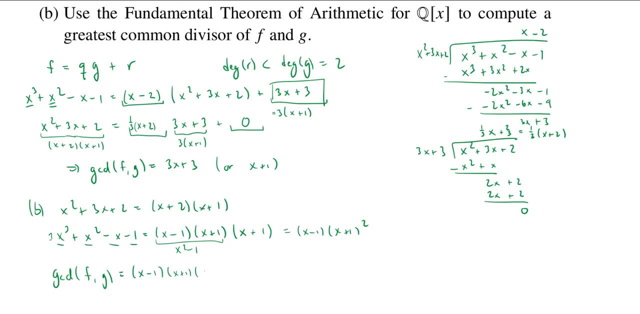 So let's write all these down: x minus 1, x plus 1,, x plus 2.. And I want to know which is the smallest exponent I see. So for x minus 1.. It occurs one time in f right. 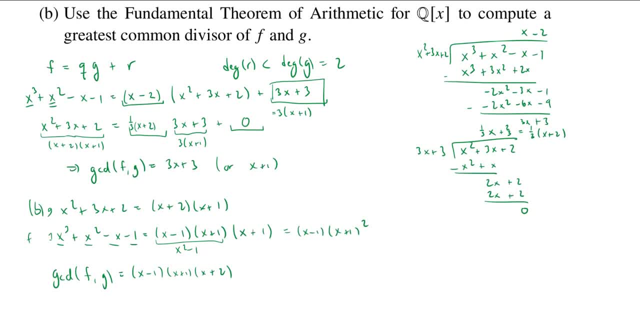 This was g up here, And it doesn't occur at all in g, which tells me that I should be using the smallest one, which is 0.. How about x plus 1?? It shows up twice in f and one time in g.